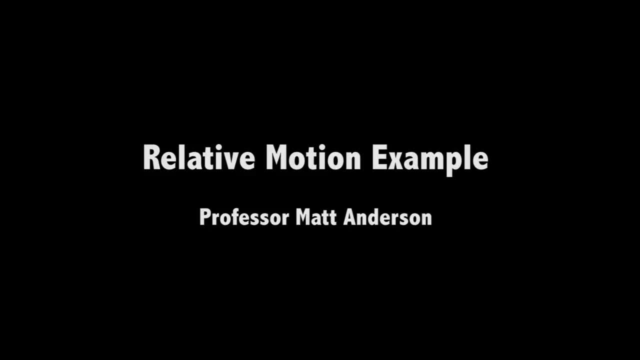 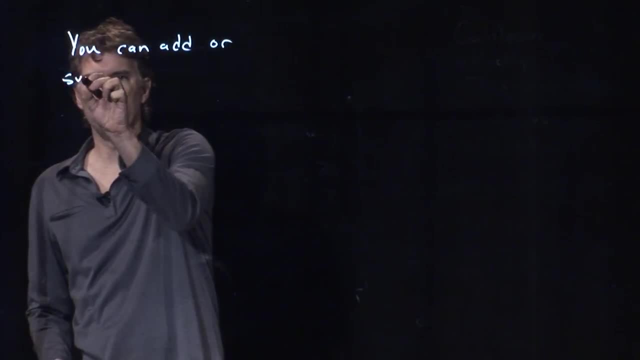 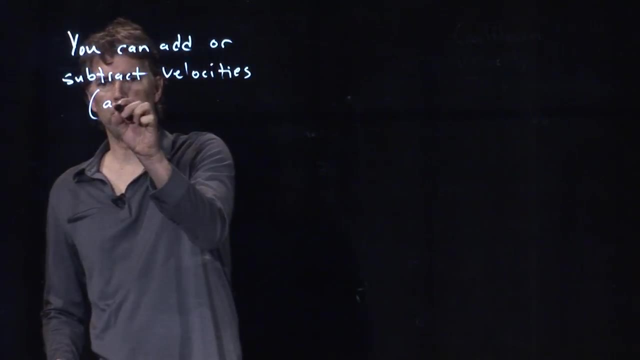 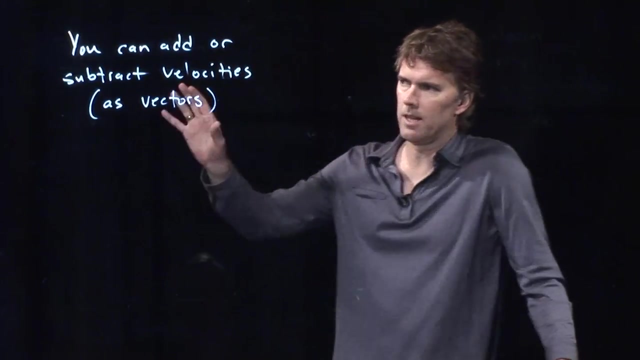 Okay, so Galileo said the following: You can add or subtract velocities, but you have to be careful and do it as vectors. Okay, so anytime we're dealing with Galilean velocity transformation, we're always talking about frames that are moving along coordinate systems. 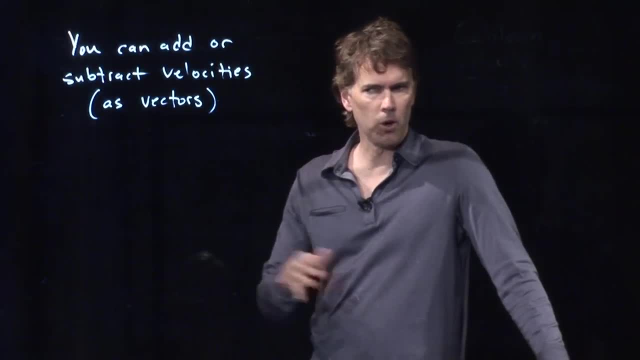 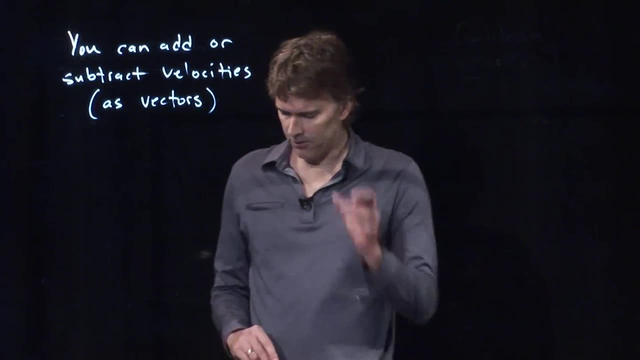 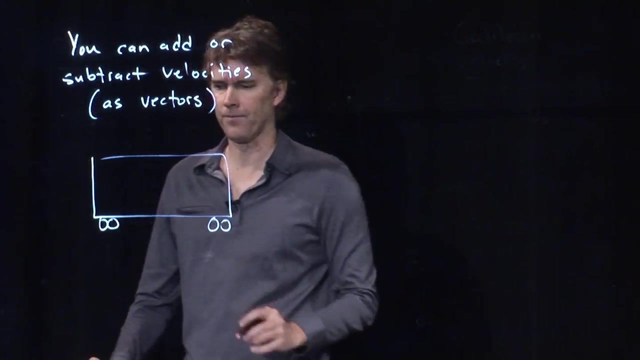 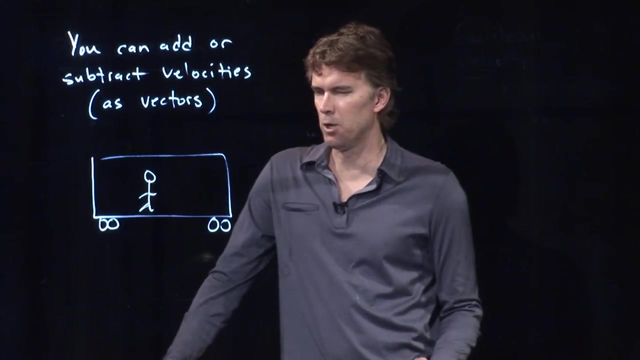 that are moving along at constant velocity. No acceleration in those frames. Okay, constant velocity motion between the two frames. So let's try the following example. Let's say that we are standing on a train and now we are walking inside that train. Okay, and you? 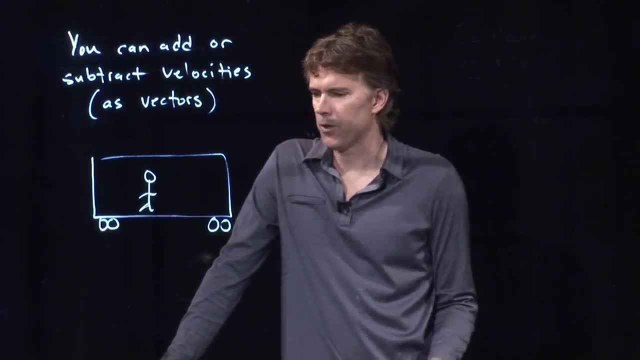 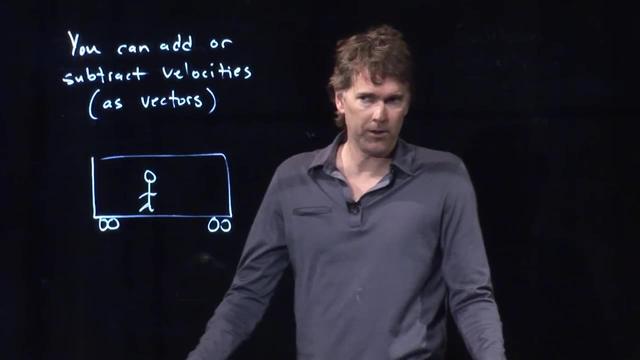 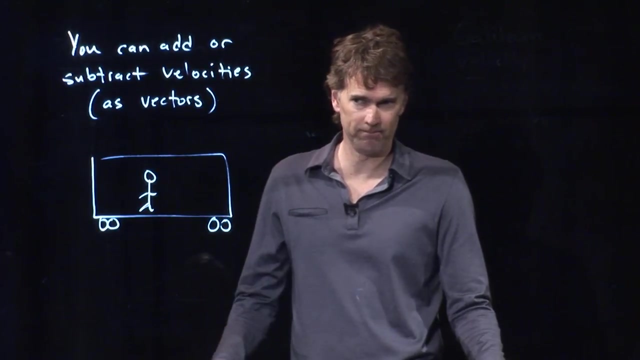 probably already know the answer to this, but if the train is moving at 30 miles per hour and I'm walking inside it at 10 miles per hour, what's the velocity of me relative to the Earth? Anybody know what that is? If you know, raise your hand. Yeah, Samantha. 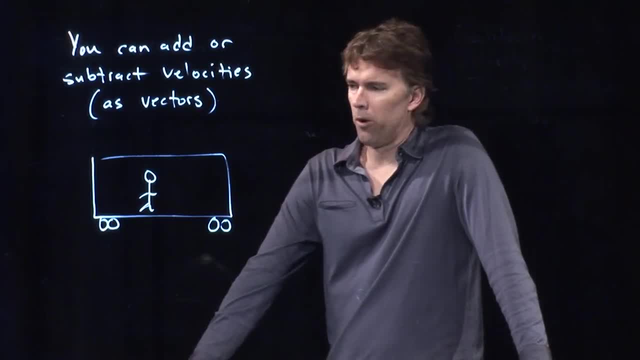 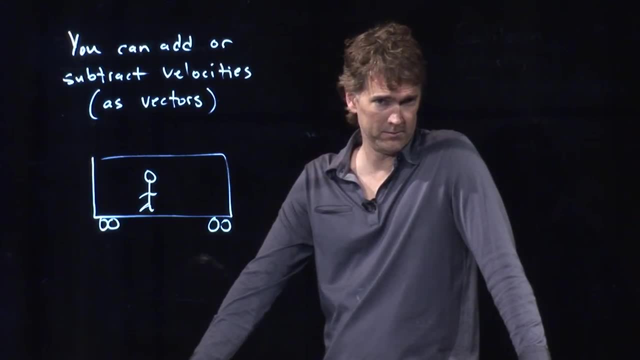 40 miles per hour. 40 miles per hour, That sounds good. Everybody else agree with that? Yes, Okay, so we're going to do the following. We're going to do that 40 miles per hour. Is there any other possible solution? Yeah, Sean, It could be. 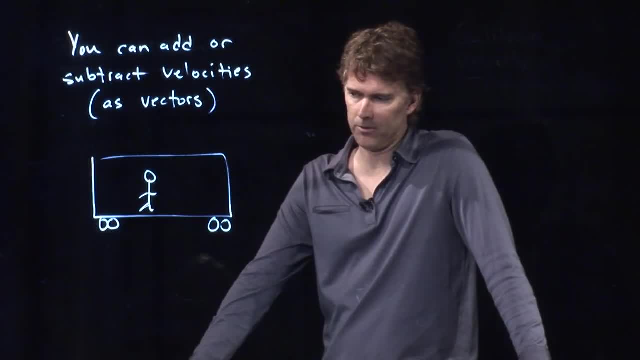 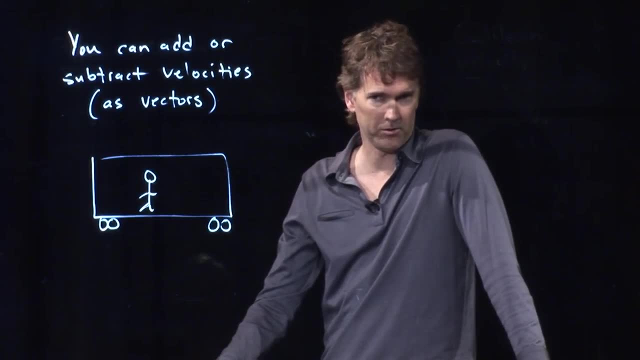 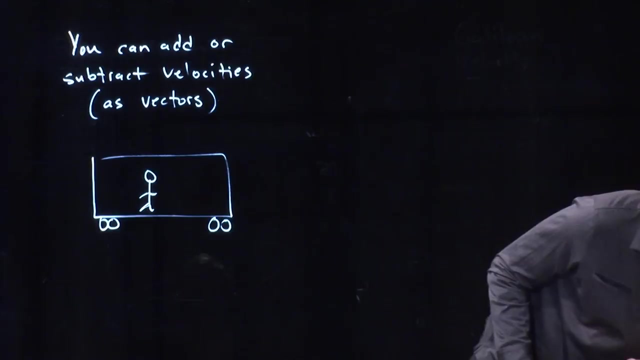 20 miles per hour. if they're walking the other direction, It could be 20 miles per hour absolutely. If I'm walking with the train's motion, it would be 40 miles per hour. If I'm walking against it, it would be 20 miles per hour. Any other possible solution? Yeah, Doug. 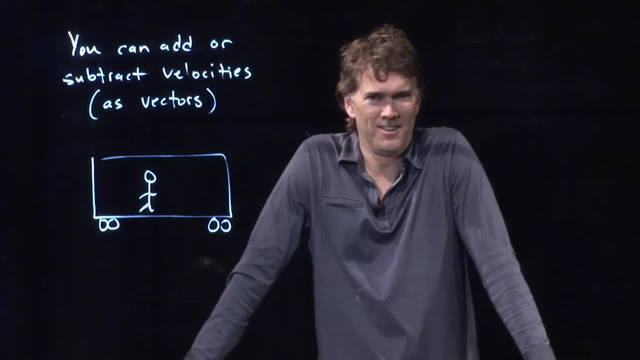 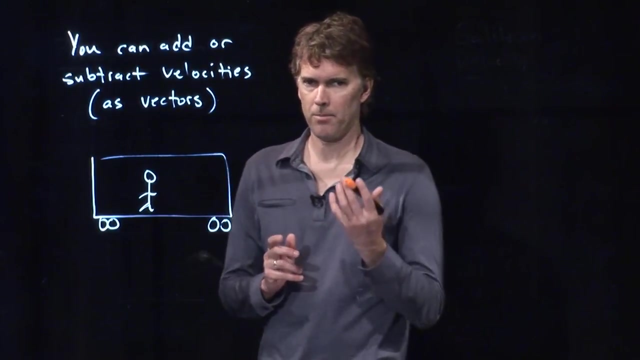 It could be the same if you're walking sideways. Okay, it could be something else if you're walking sideways, Maybe not the same as the train or the same as you, but something else. So the idea is that we're going to add up vectors, Okay, and let's identify what those 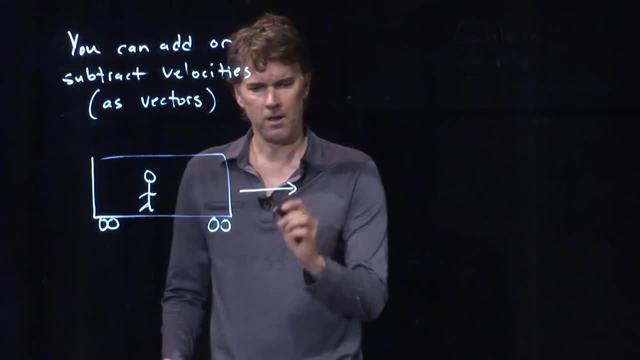 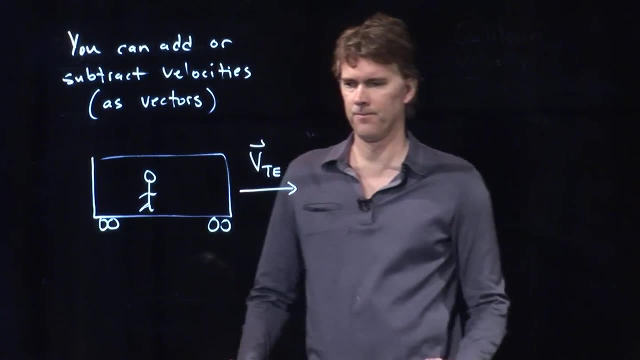 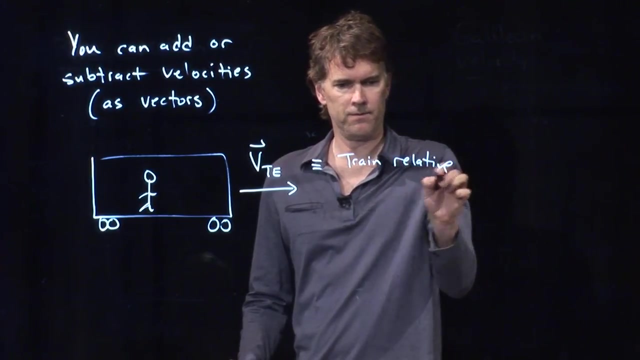 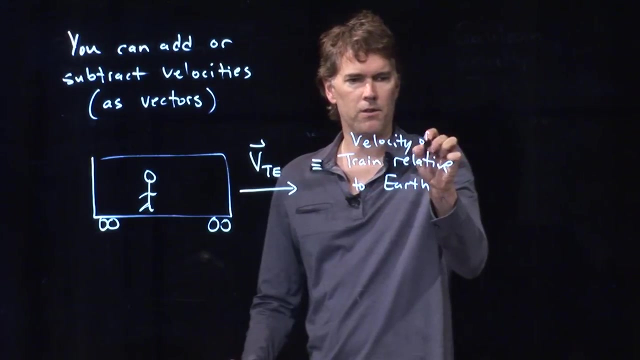 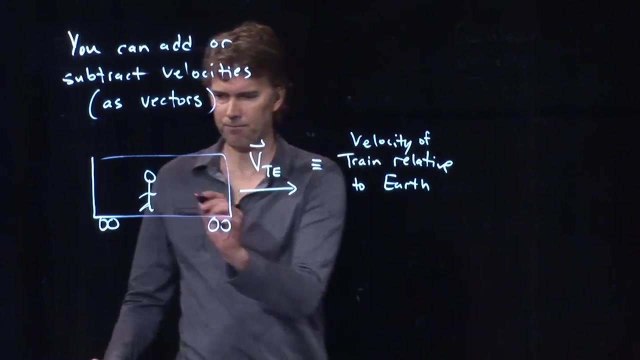 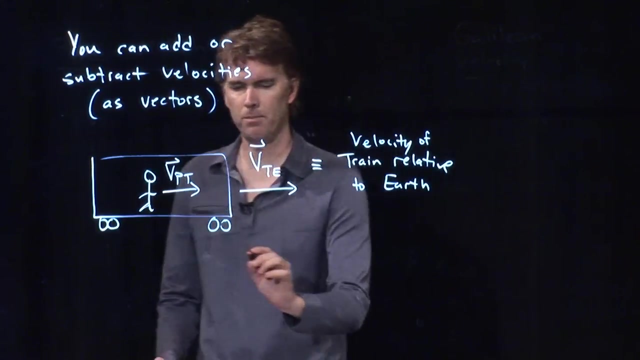 vectors are. So we have the vector for the velocity of the train relative to the Earth. Okay, this is train relative to Earth And specifically, it's the velocity of the train relative to Earth. And now we have a velocity of the person relative to the train. Okay, 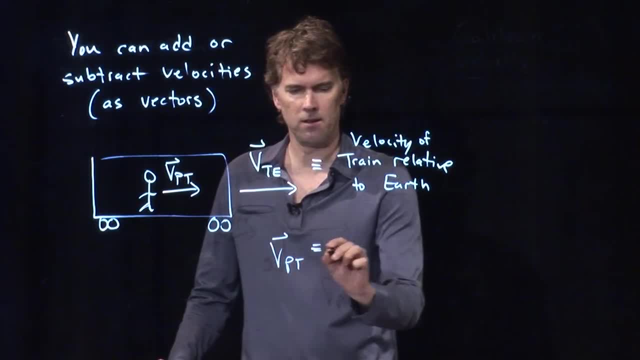 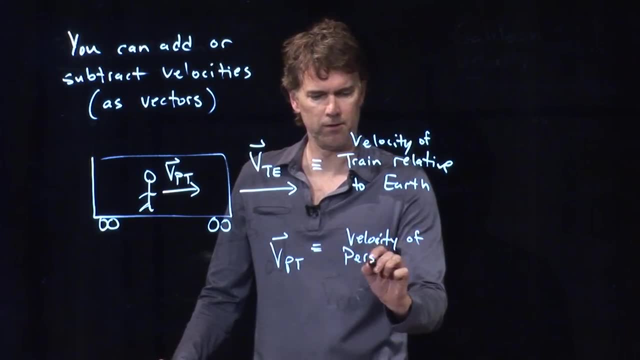 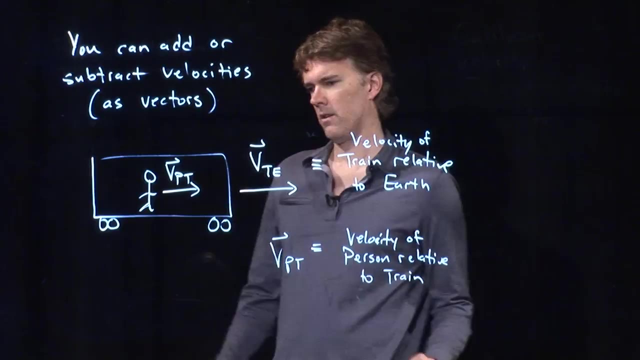 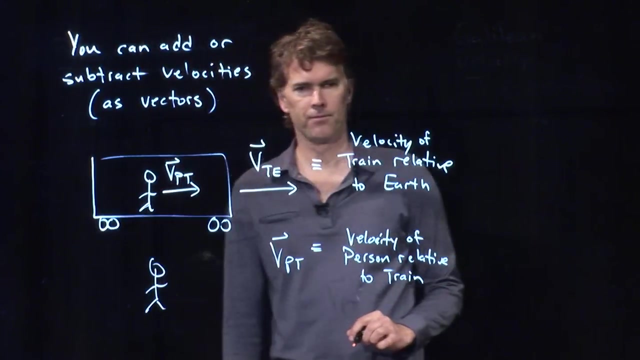 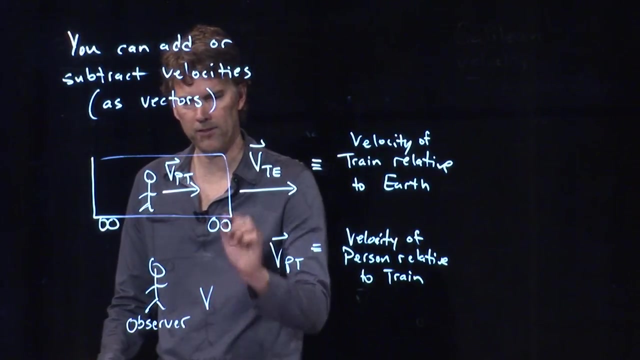 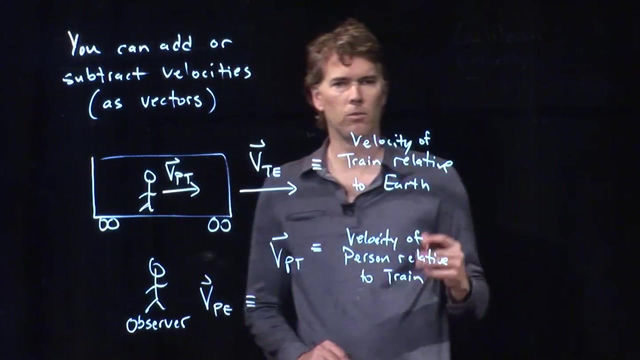 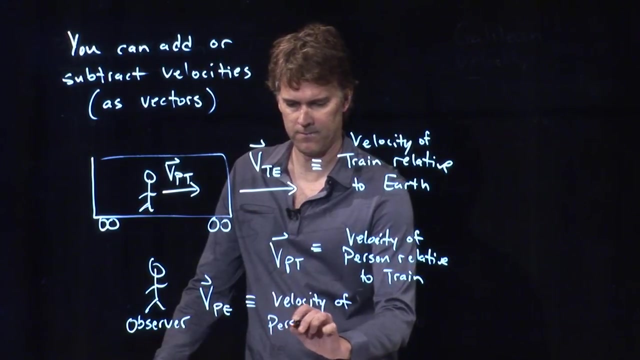 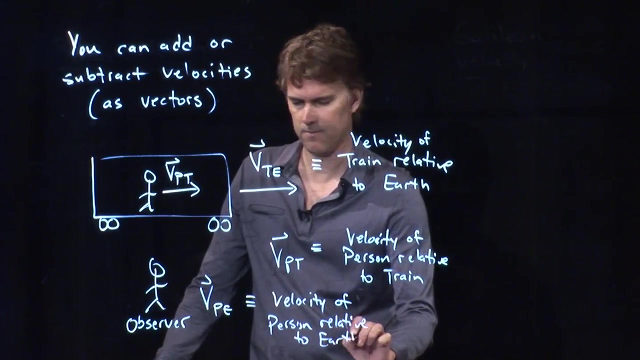 but what we really want to know is: what does somebody out here observe? Okay, this is the observer in the stationary frame, And they're going to say, oh, the velocity of that person relative to the Earth is what? And what is the velocity of the person relative to the Earth? 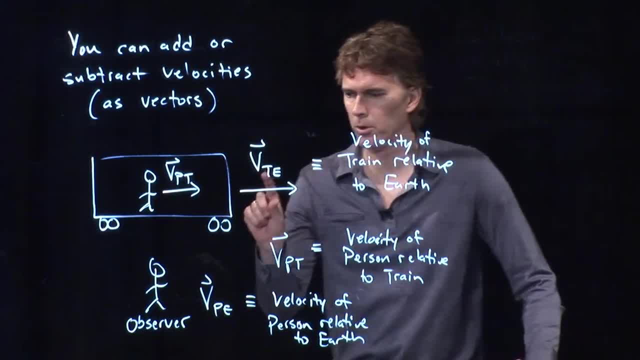 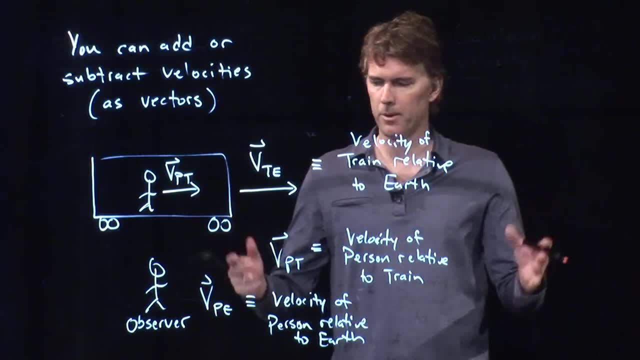 Okay, So what we said was, if the train's moving at 30 miles per hour and you're walking at 10 miles per hour, then we could be moving at 40 miles per hour relative to the Earth, But we could be walking the other way, and then it would be 30 minus 10, which would 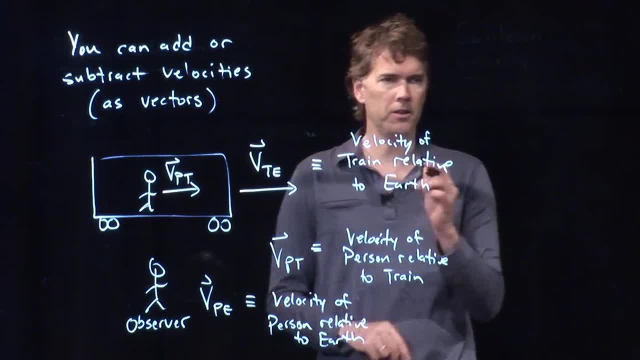 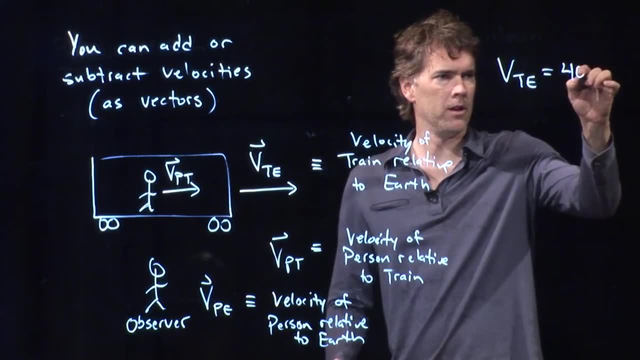 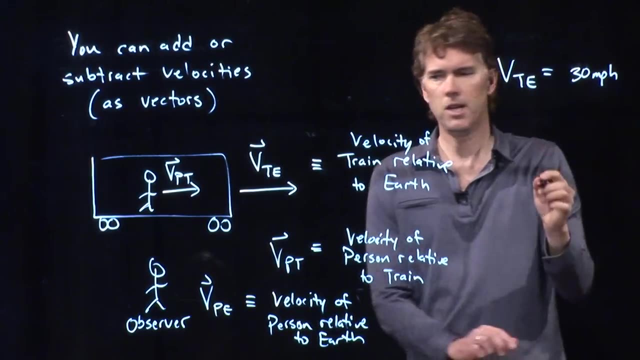 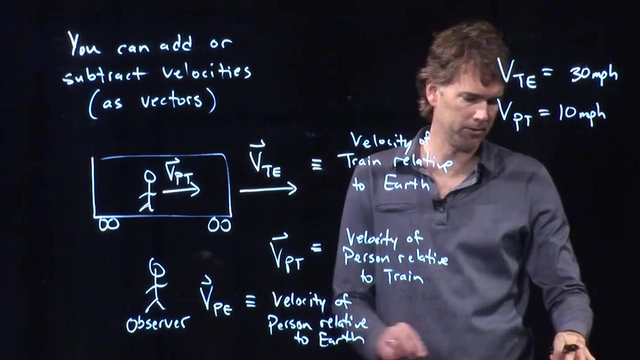 be 20 miles per hour relative to the Earth. So let's put the bounds on it like that. Let's say that the speed of the train relative to the Earth is- what did we say? 30 miles per hour, 30 mph, And the speed of the person on the train is 10 miles per hour. Maybe faster. 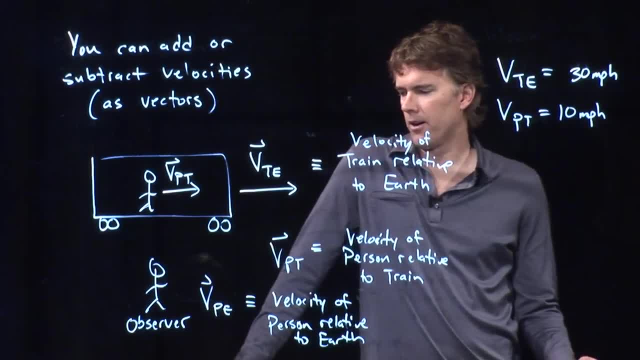 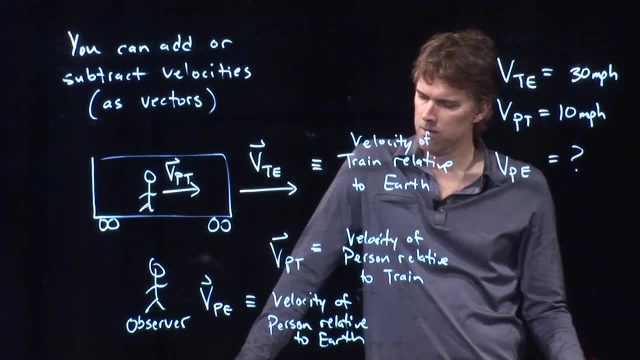 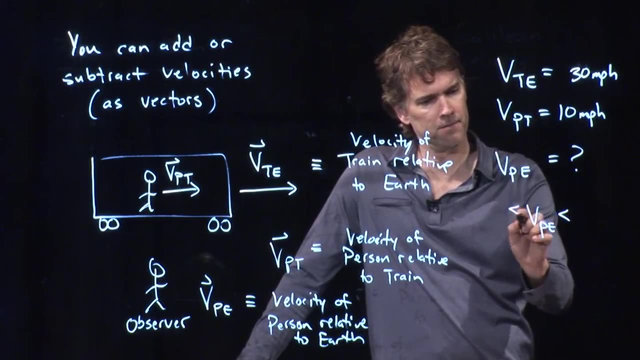 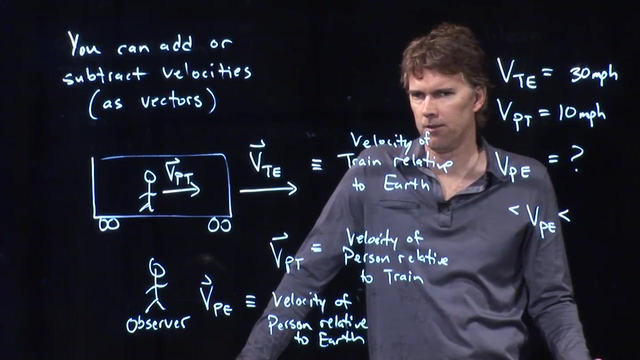 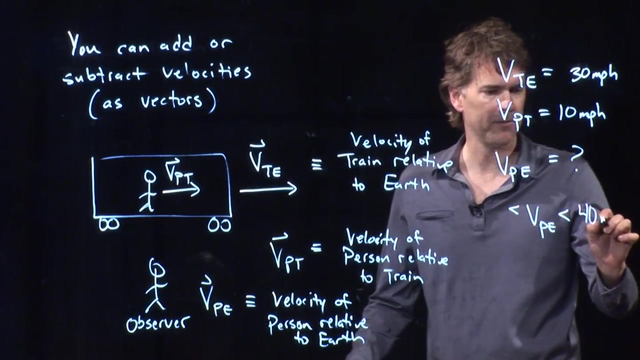 than a walk, more like a run. And now we need to figure out VPE. What is the biggest that VPE could be? We already said the answer to this right: It's if you're walking in the same direction as the train's moving. The biggest it could be is 40.. What about the smallest it could? 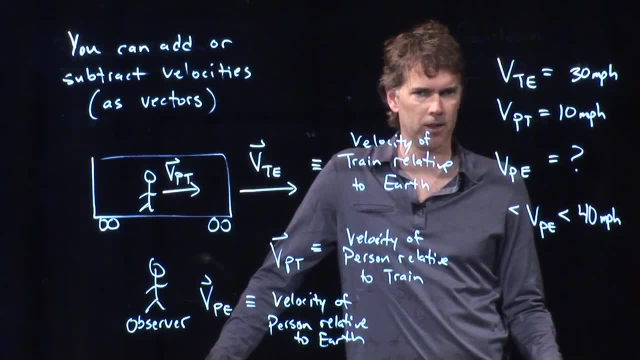 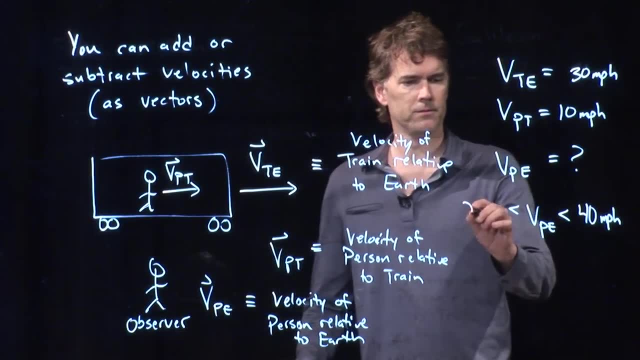 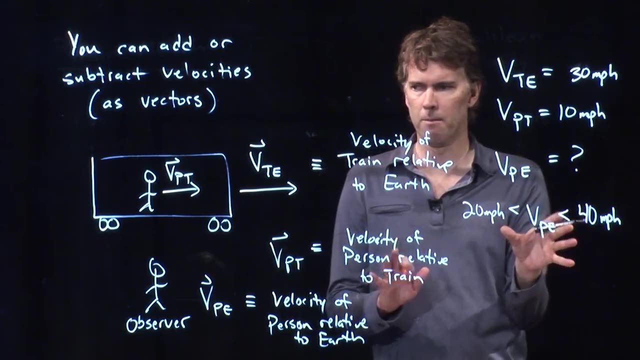 be. Anybody have a thought on that? Yeah, Ian, 20 miles per hour. 20 miles per hour, Yeah, Yeah. Okay, Those are the bounds on VPE. This already makes sense to you, but let's put it in the. 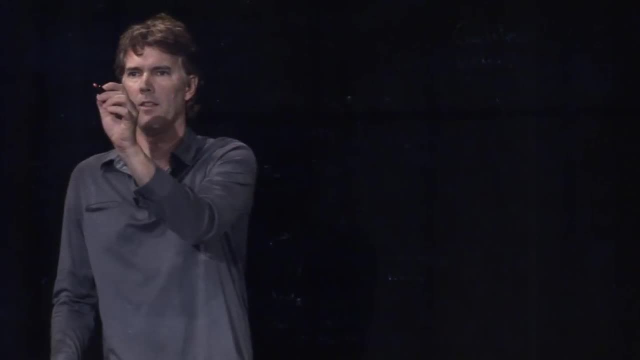 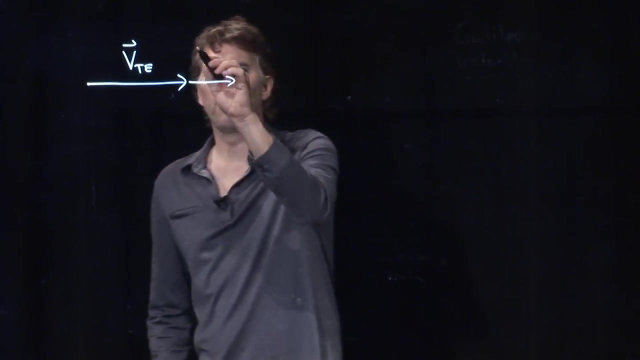 context of vectors. Okay, we said that the train is doing this. This is V of the train relative to the Earth. If I add to that the vector of the person relative to the train, then I just do a tip-to-tail method. 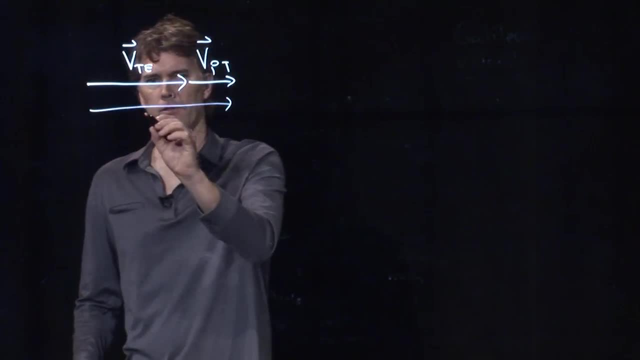 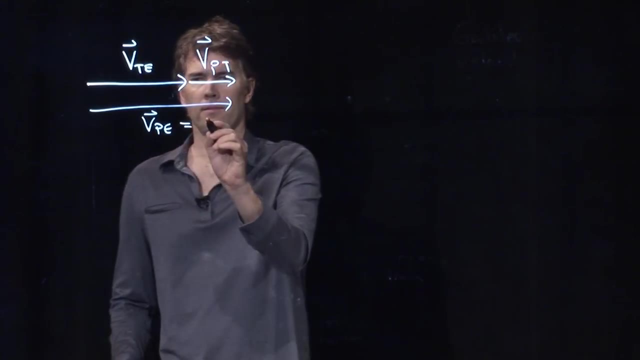 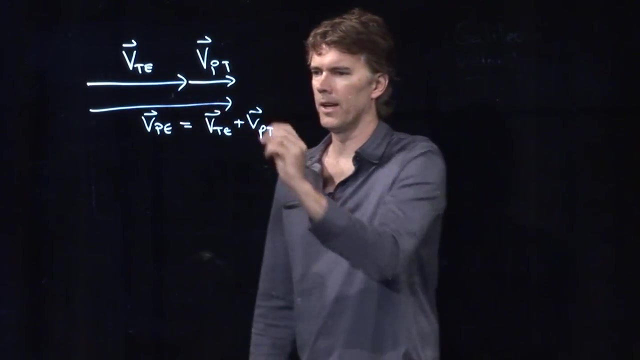 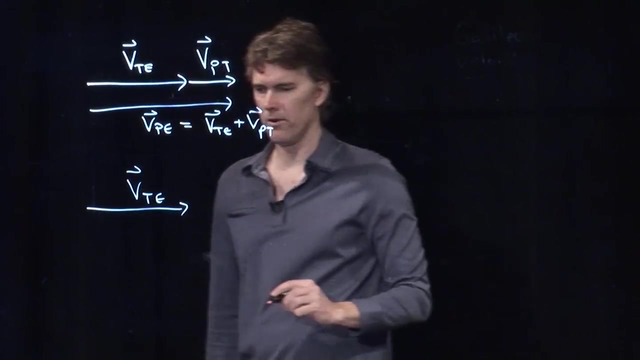 And I add those two vectors up and I get the velocity of the person relative to the Earth. Okay, But what about when I go the other way? If I'm going the other way, then the velocity of the train relative to the Earth I have to add a negative to the velocity of the train. 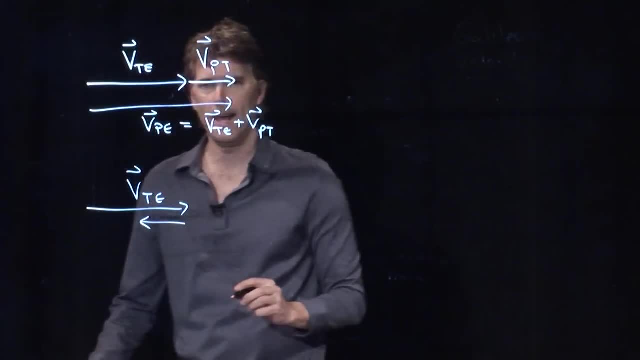 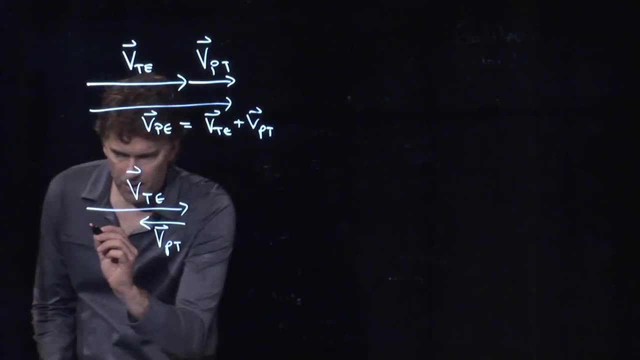 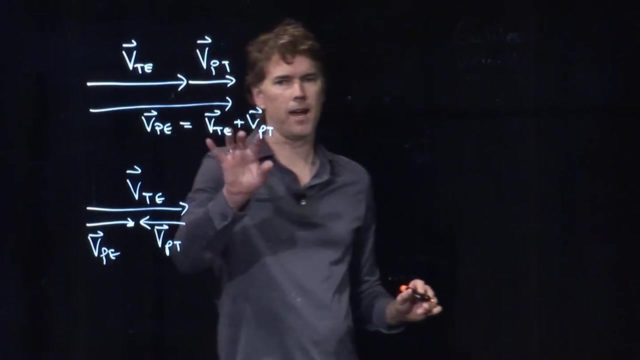 Okay, Okay, Okay, Okay. So that will be a positive Velocity of the person relative to the train And therefore the sum is going to be that little bit right there. Okay, So in that case we're going to get 40 miles per hour. In this case, we're going to get 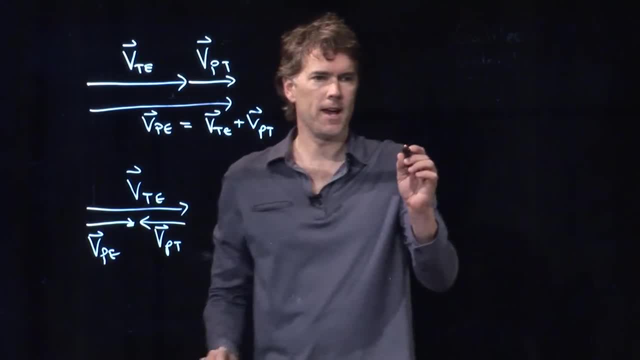 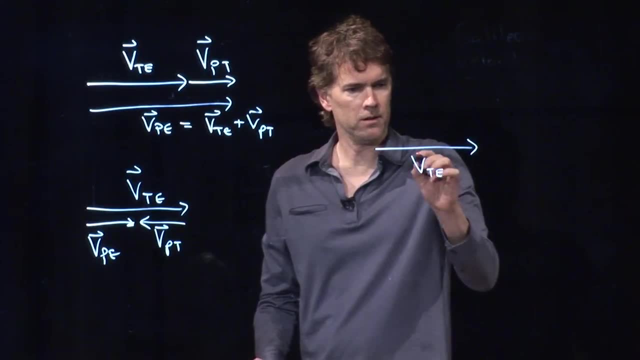 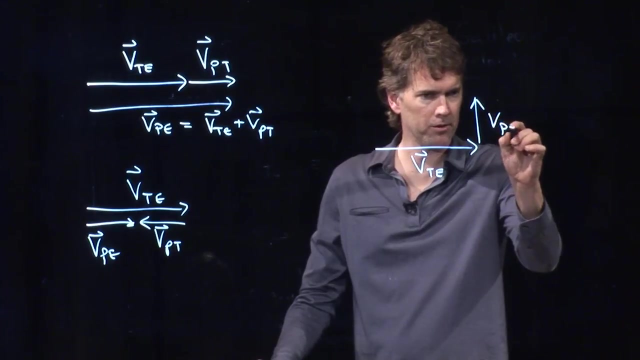 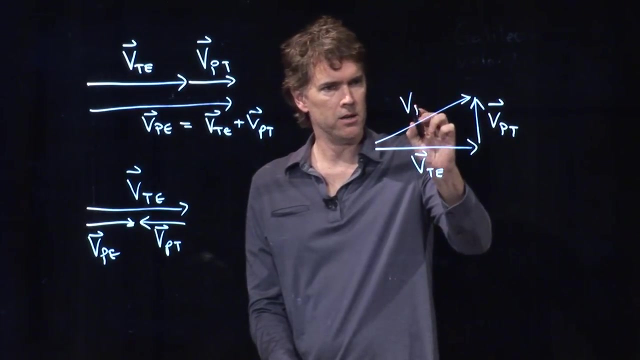 20 miles per hour, But of course we don't have to add those vectors in the same direction. You could be sideways relative to the train, and so this would be the person relative to the train, and therefore the sum of those two is right there. this is the person.